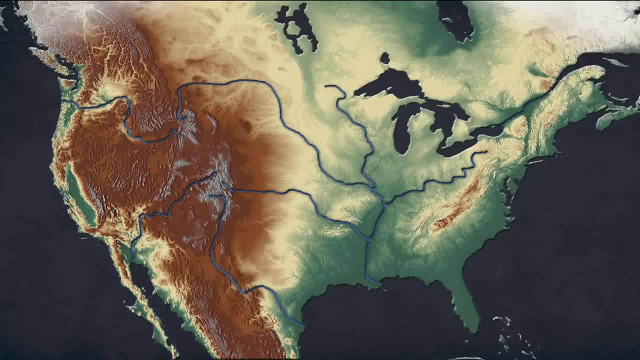 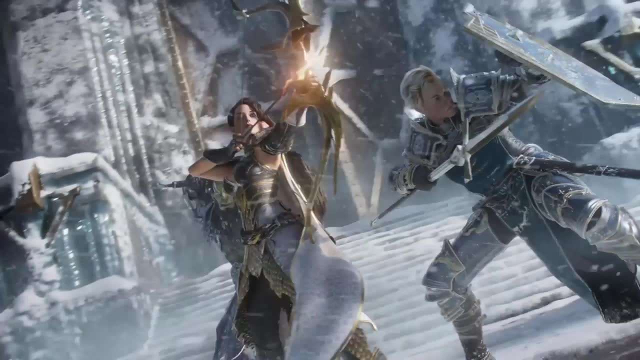 ended and the land bridge became submerged by the rising ocean. But before we move any further, we want to give a big thank you to Raid Shadow Legends for sponsoring this video. Raid is a brand new RPG game that you will definitely enjoy. The game has an amazing storyline. 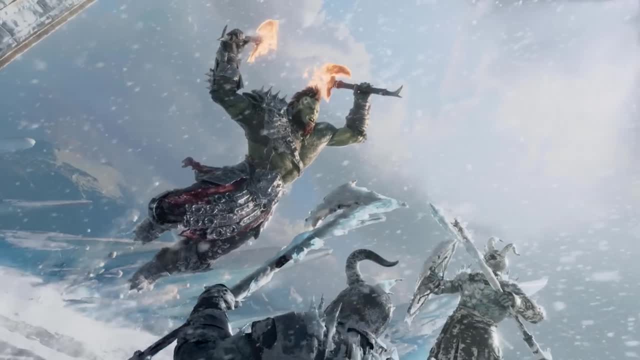 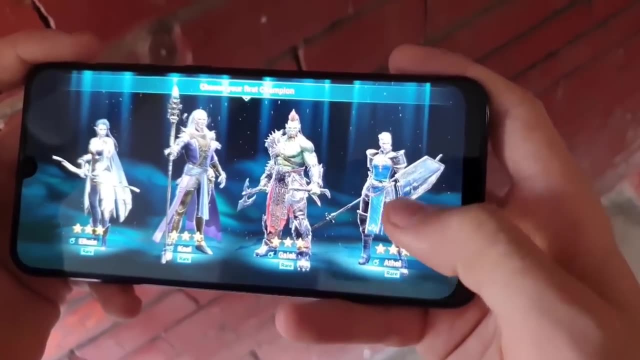 great looking 3D graphics, incredible boss fights and PvP battles. You can choose from hundreds of champions to collect and customize as you wish. I personally prefer Ethel because of her great skills and the way she looks. She is not the only awesome champion, but in my opinion you should definitely. 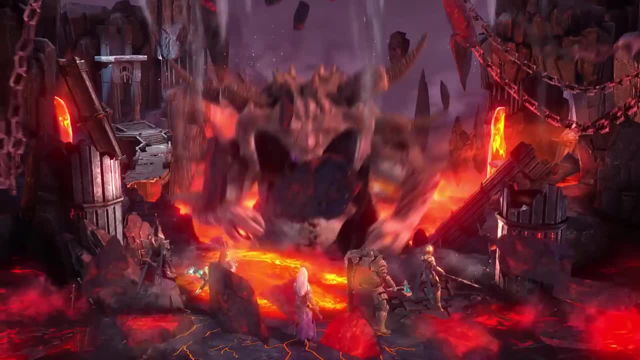 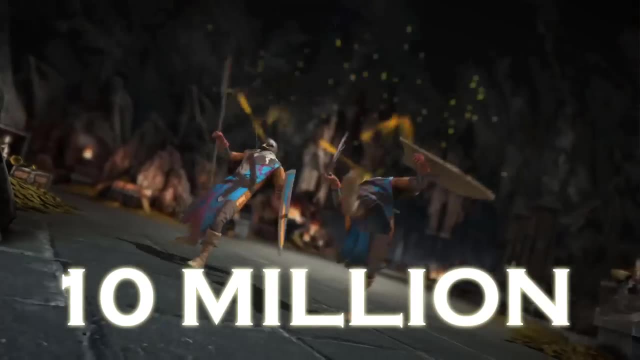 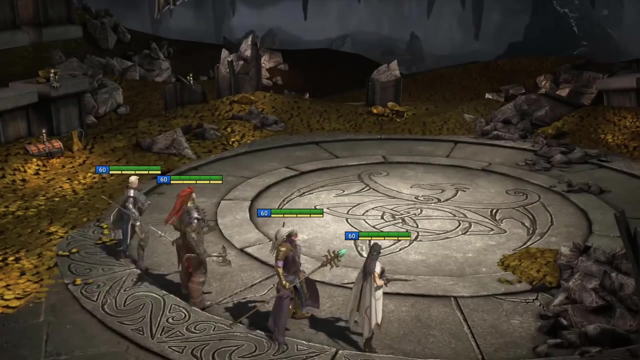 try her out. Raid is a rapid growing game attracting more and more players every day. By now, 10 million players worldwide have already downloaded the game in less than six months. The game is consistently updated, so you will not get bored playing it. After downloading the game, I can surely say that I am impressed by its 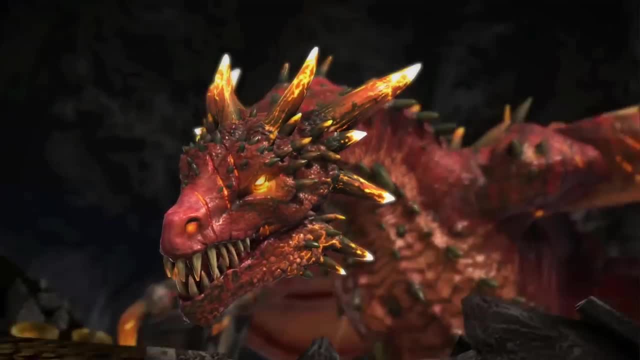 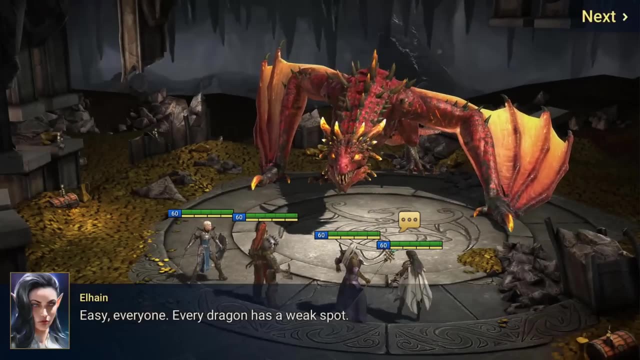 quality and graphics. Playing Raid is the most immersive experience you will find on a smartphone, and it can only really be compared with the biggest PC and console titles. And the best part of all of this, it's totally free. With 300,000 reviews, Raid has almost 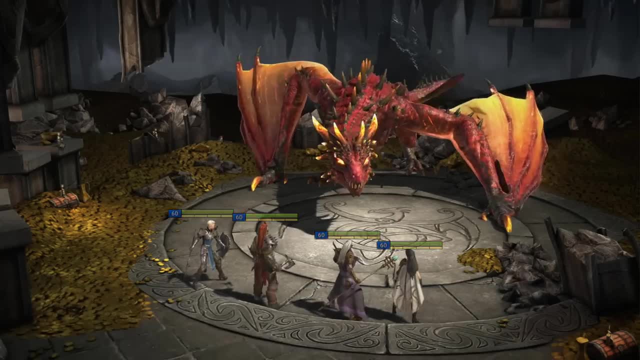 a perfect score on the Play Store. This proves just how amazing the game is, So be sure to click on our special link in the description to get 50,000 silver and an epic champion for Raid. Thanks for watching and I'll see you in the next video. 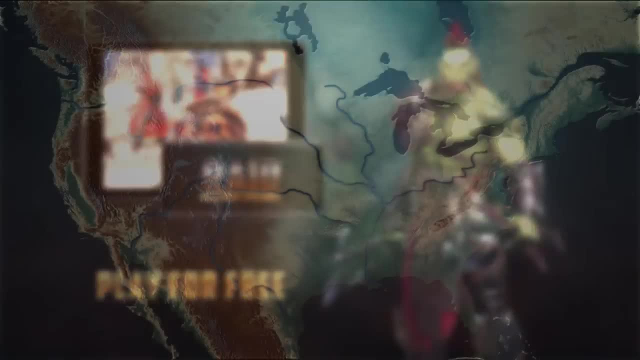 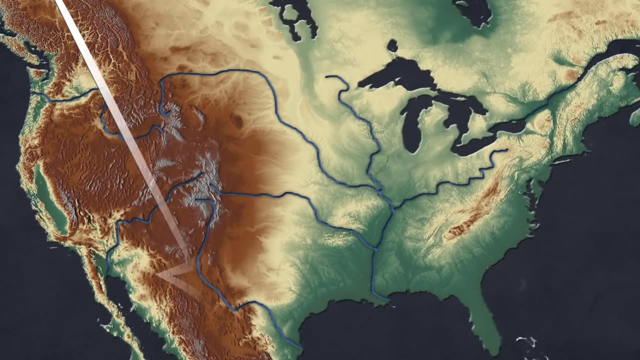 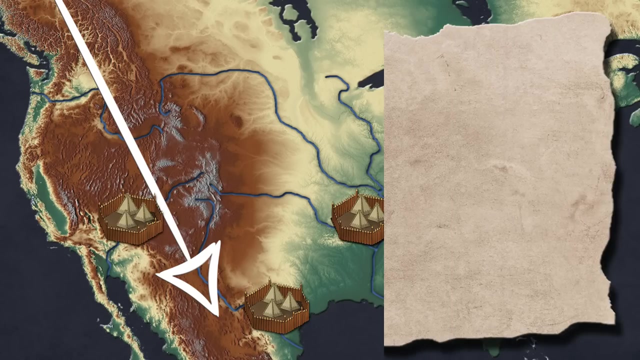 The early inhabitants were called the Paleo-Americans. In time they migrated even deeper in Americas and they formed tribes and nations. They created interesting civilizations, developing their own culture. Among the cultures that existed here we can mention Adena culture Iroquois. 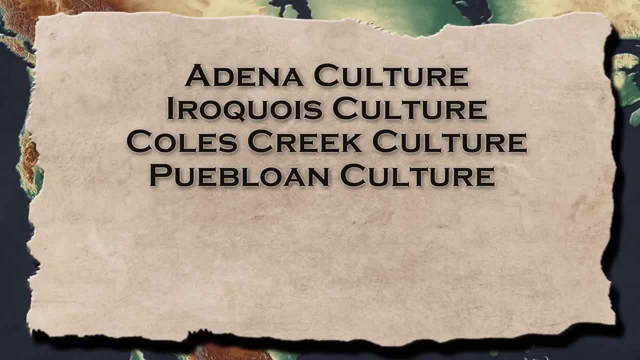 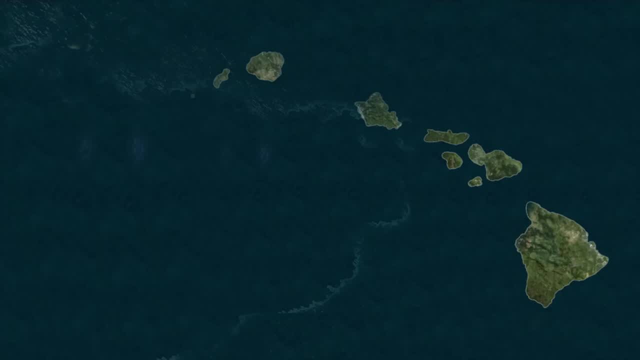 culture, Coles Creek culture, Puebloan culture and Mississippian culture, But another part of today is the American culture. The United States has an interesting and different history. Speaking about Hawaii, this land wasn't inhabited until the first centuries AD. Native development started with. 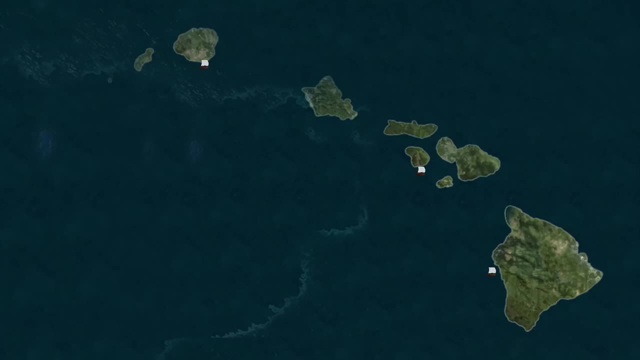 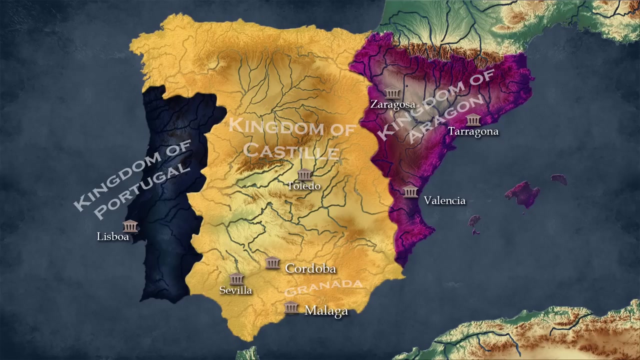 the settlement of Polynesian people between the 1st and 10th centuries, Starting in the 15th century. European colonization began In 1492, a Spanish expedition headed by the Italian explorer Christopher Columbus sailed west to find a new trade route to the Far East, but landed in what? 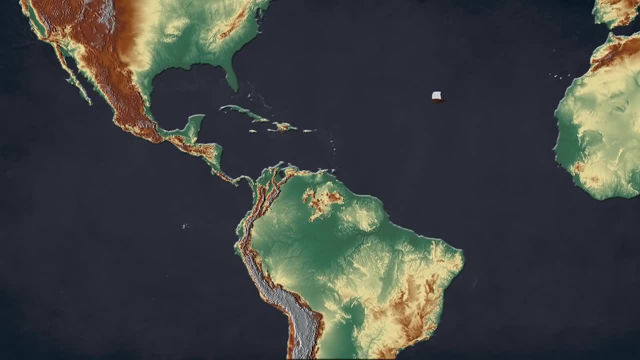 came to be known to Europeans as the Pueblo. The Pueblo was a small town in the middle of the Far East. After this event, in the next decades, more and more ships sailed west to establish colonies and trade posts. The Spaniards began building their American empire. 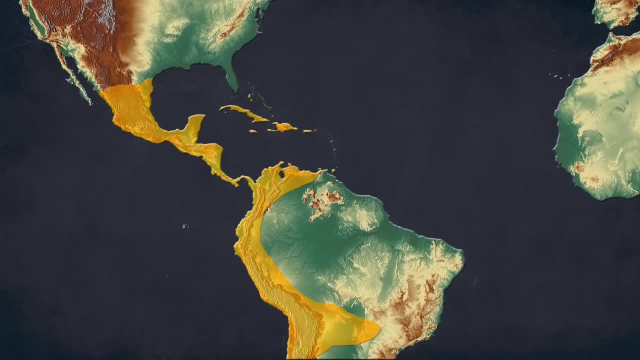 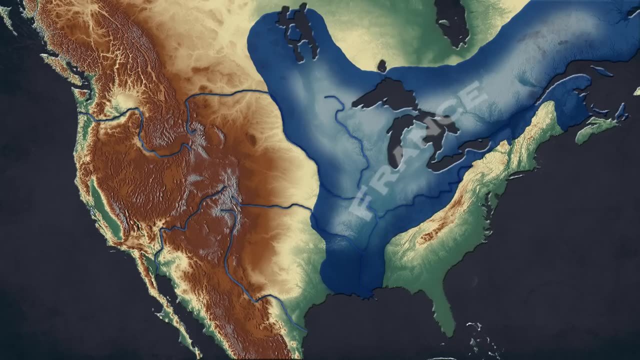 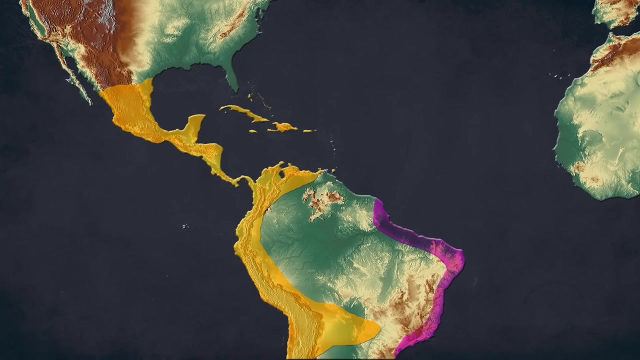 using islands such as Cuba, Puerto Rico and Hispaniola as bases, They expanded hugely. France founded colonies in eastern North America, a number of Caribbean islands and small coastal parts of South America. Portugal colonized Brazil. The eastern sea coast was settled primarily by the. 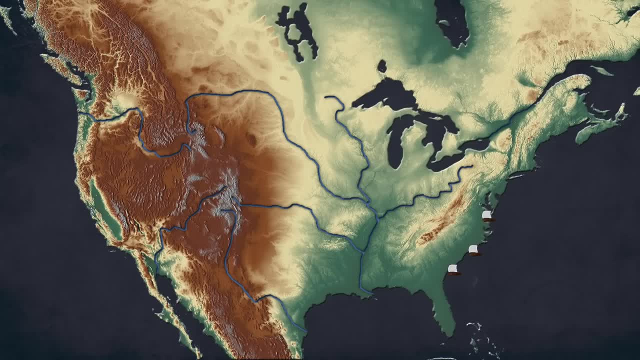 English colonists in the 17th century, along with a much smaller number of Dutch and Swedes. The first successful English colony, Jamestown, was established in 1607 on the James River in Virginia. New wave of settlers arrived in the late 17th century and established commercial. 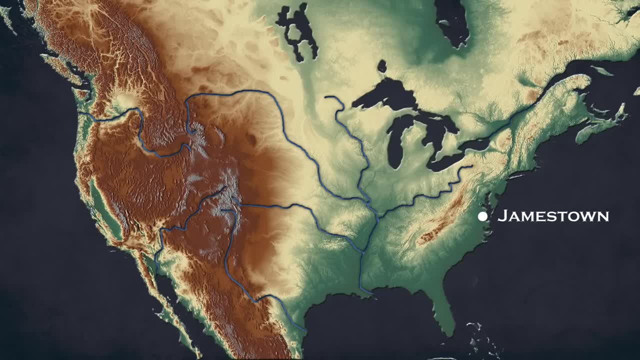 agriculture based on tobacco. Even though there were some conflicts between the Native Americans and English settlers, the colonies managed to expand pretty fast and more and more people settled in. The 13 American colonies had slightly different governmental structure. In fact, a colony was: 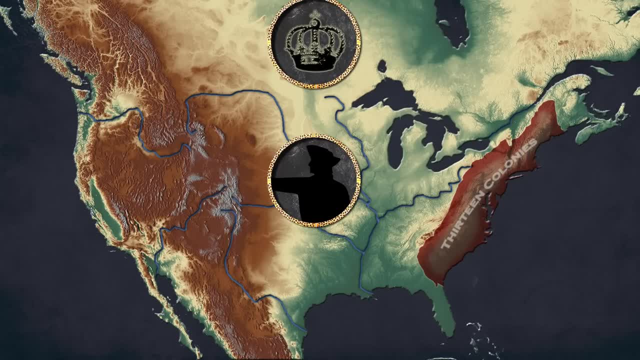 ruled by a governor appointed from London. This governor controlled the administration and relied upon a locally elected legislature to vote taxes and make laws. By the 18th century, the American colonies were growing very rapidly and, as a result of low death rates, along with ample supplies of 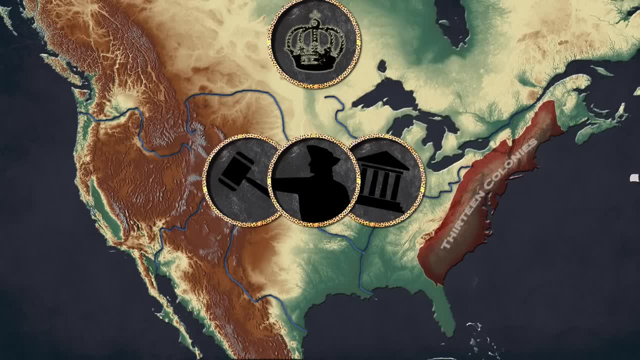 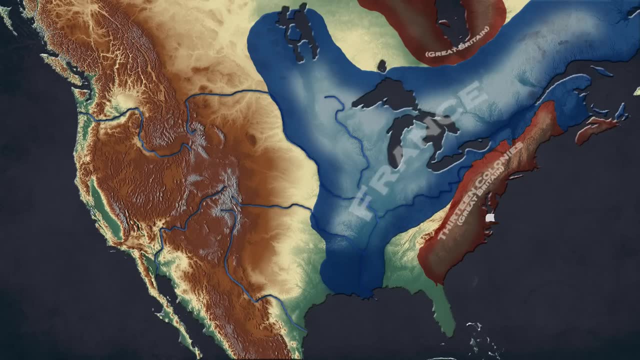 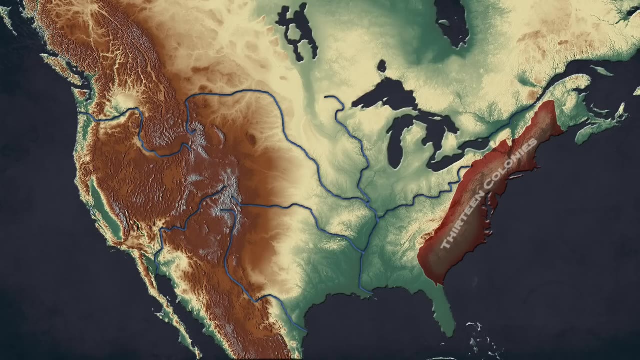 land and food. this attracted a heavy flow of immigrants. The tobacco and rice plantations in the 18th century imported African slaves for labor from the British colonies in the West Indies, And by the 1770s African slaves compromised a fifth of the American population. The question 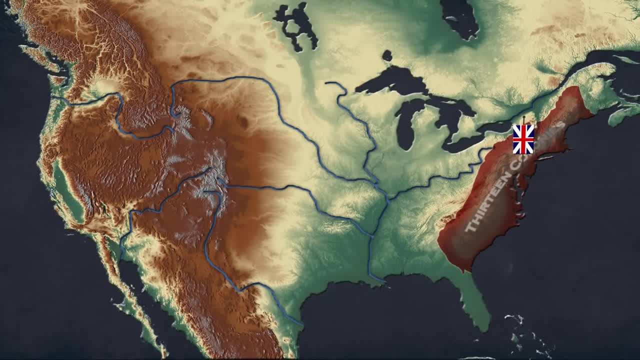 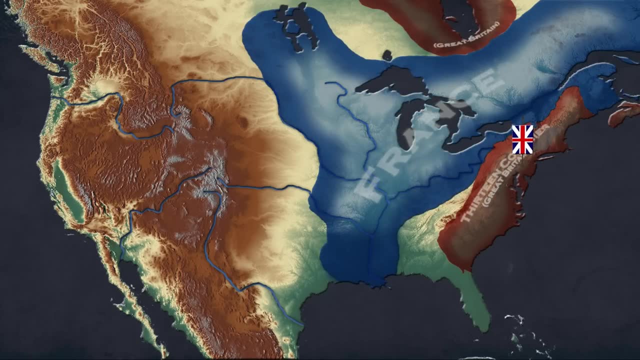 of independence from Britain did not arise as long as the colonies needed British military support against the French and Spanish powers. The French and Indian War was an event created by the political development of the colonies. It was also part of the larger Seven Years War. 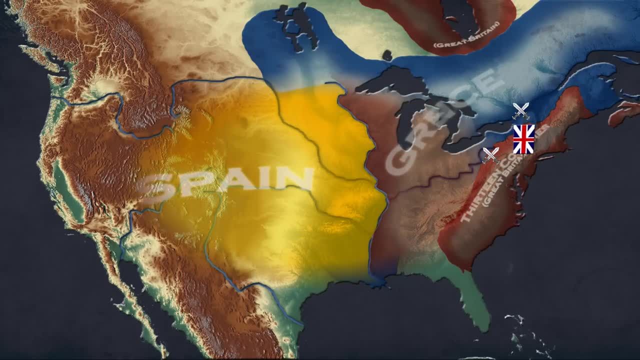 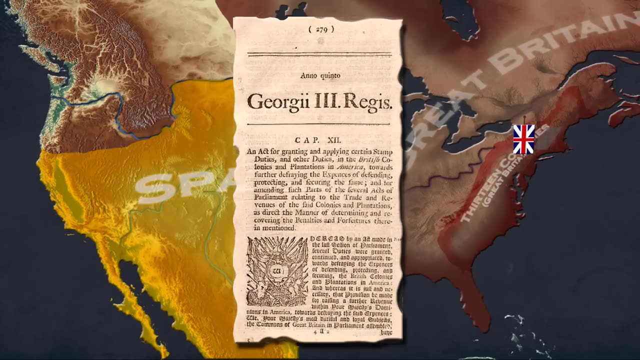 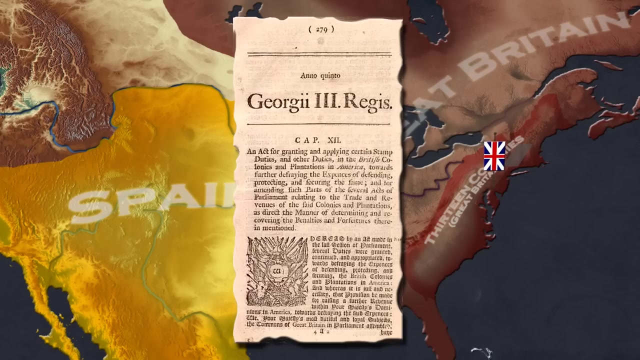 Britain beat French forces and France lost their colonies in territories in Canada and Louisiana. The war was costly and Britain needed money. The British Parliament passed the Stamp Act of 1765, imposing a tax on the colonies without going through the colonial legislatures. The issue was drawn: Did Parliament have this right to tax? 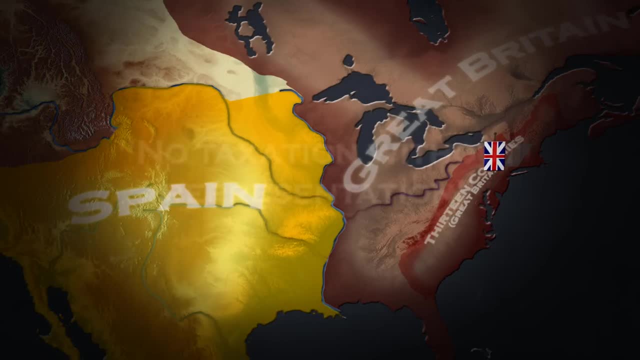 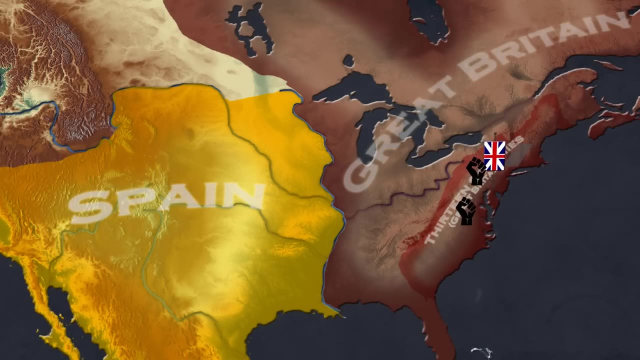 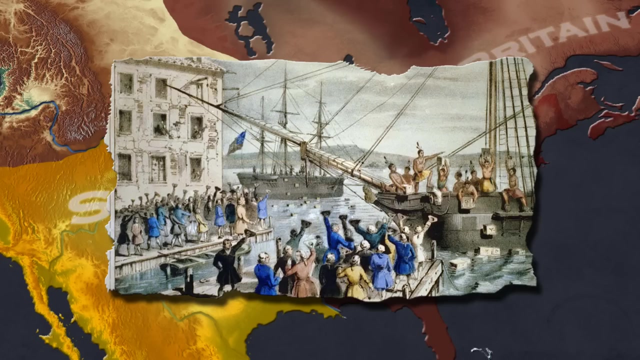 Americans who were not represented in it, Crying no taxation. without representation, The colonists refused to pay the taxes as tensions escalated in the late 1760s and early 1770s. The Boston Tea Party in 1773 was marked as the start of the revolution. It happened in the town. 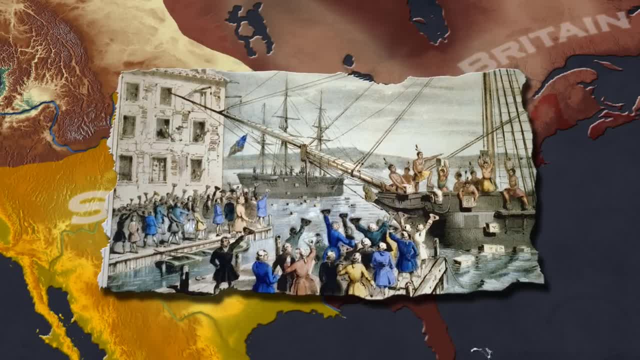 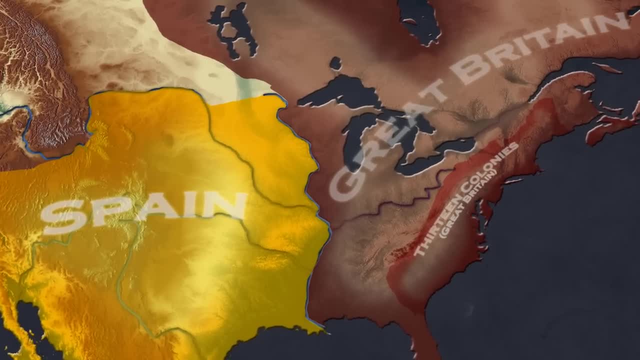 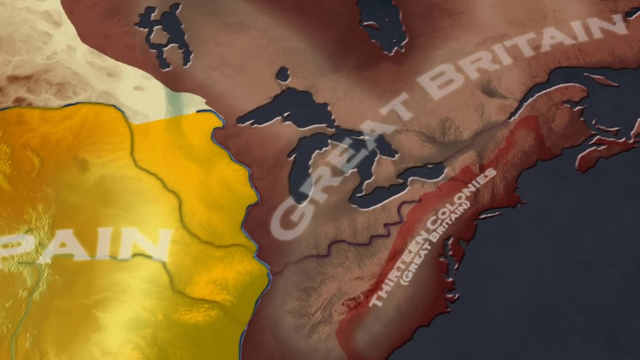 of Boston to protest against the new tax on tea. Parliament quickly responded the next year with the coercive acts stripping Massachusetts of its historic right of self-government and putting it under army rule, which sparked outrage and resistance in all 13 colonies. Leaders from all 13 colonies gathered and created the First Continental Congress. 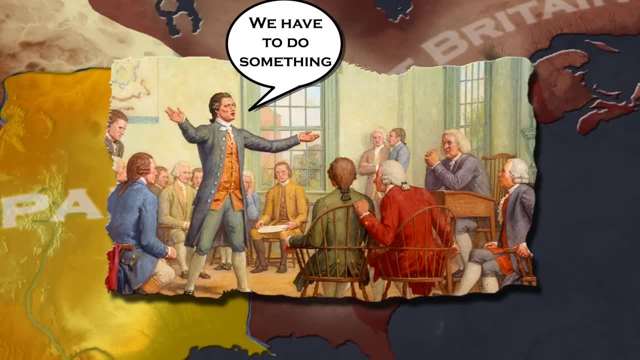 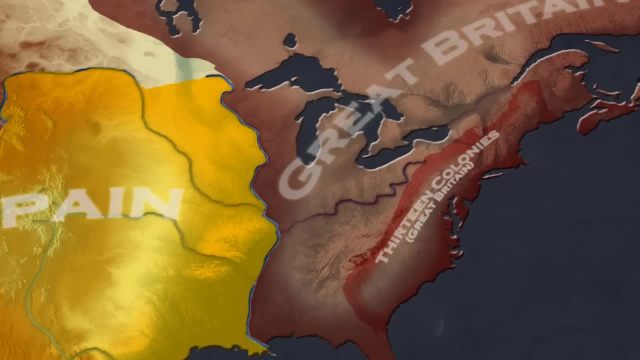 to coordinate their resistance, The Congress called for a boycott of British trade, published a list of rights and grievances and petitioned the king for redress of those grievances. It wasn't about independence at that point, But this appeal had no effect. 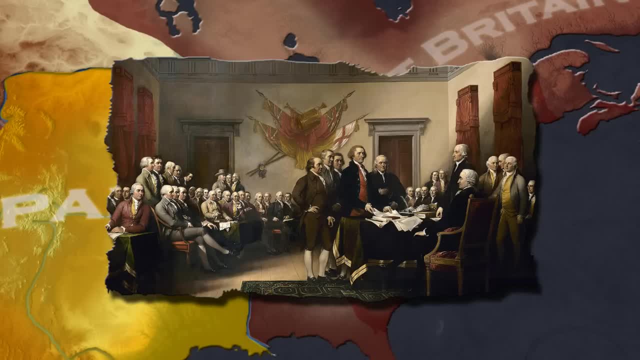 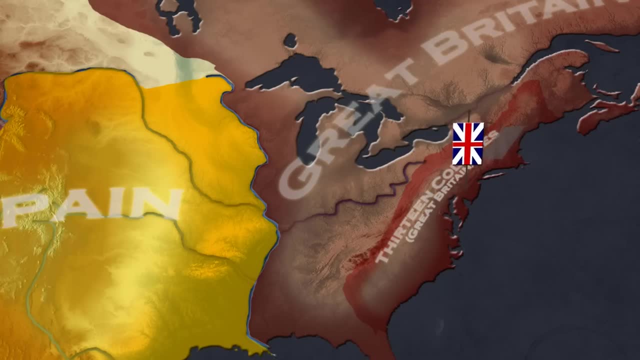 and so the Second Continental Congress was created in 1775 in order to organize the defense of the colonies against the British army. The 13 colonies began a rebellion against British rule in 1775 and proclaimed their independence in 1776 as the United States of America In the American 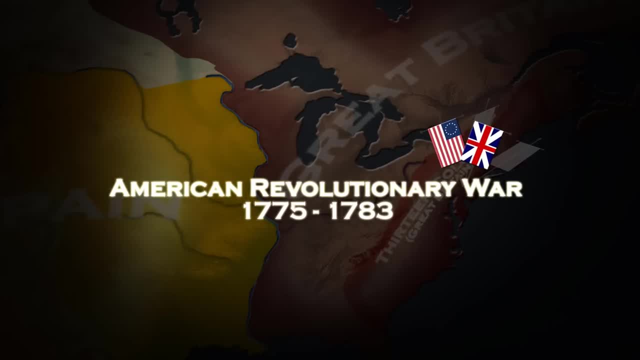 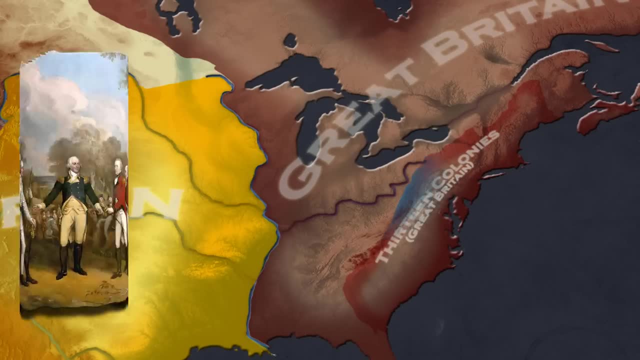 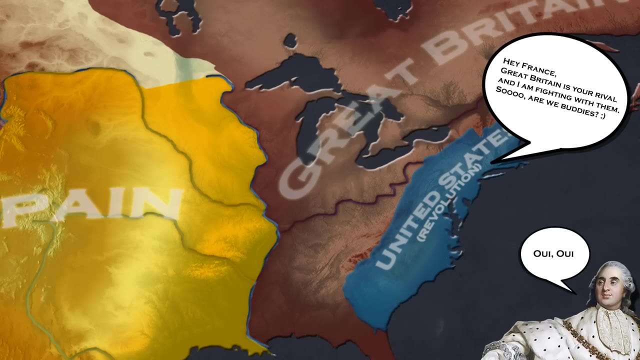 Revolutionary War. the Americans captured the British Invasion Army at Saratoga in 1777, secured the Northeast and encouraged the French to make a military alliance with the United States. France brought in Spain and the Netherlands, thus balancing the military and naval forces on each side, as Britain had no allies. 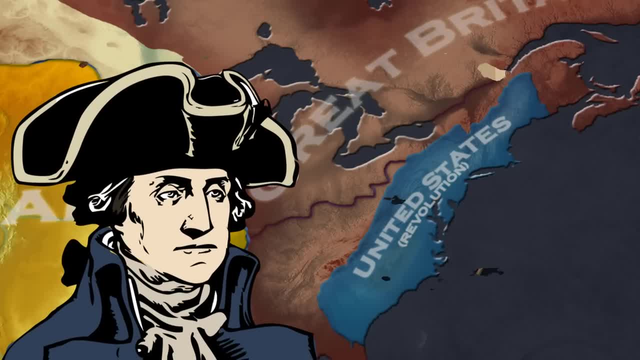 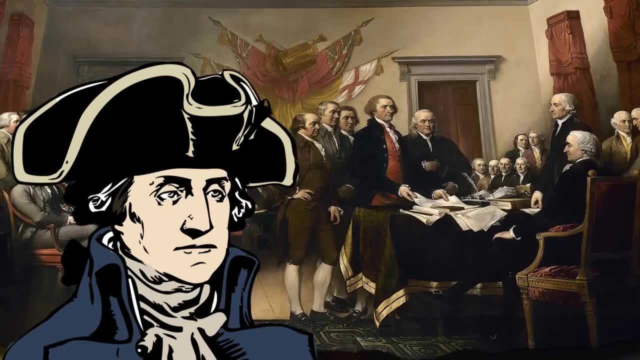 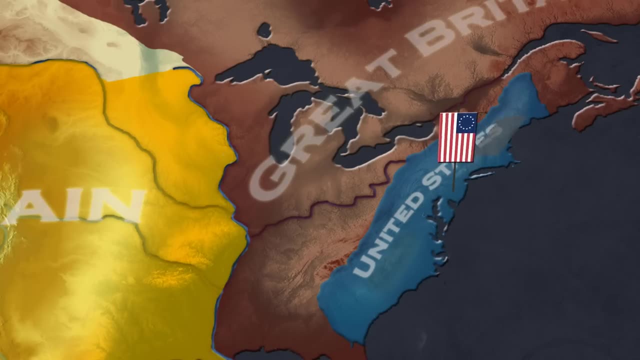 General George Washington was an excellent organizer and administrator who worked successfully with Congress and the state government. The American Revolution was a success and at the Peace of Paris of 1783, their independence was recognized. And even so, the former colonies gained more than expected. 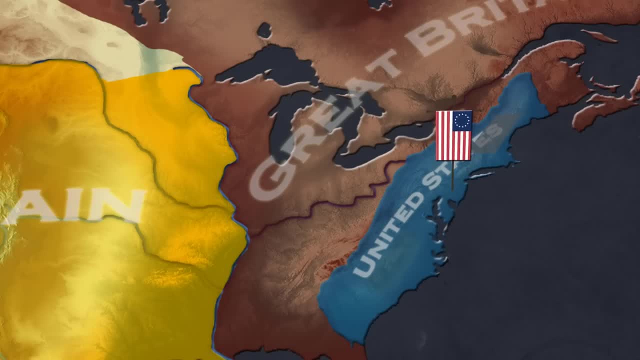 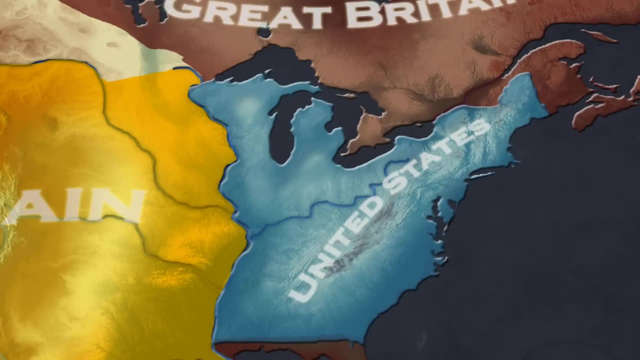 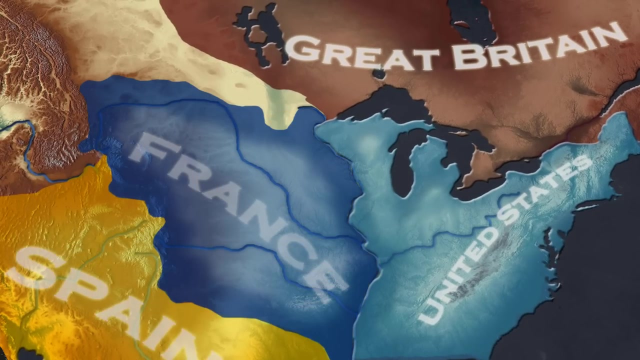 The expansion to the West started, incorporating the Amerindian lands west of the Appalachian Mountains. A deal was made by the United States president, Thomas Jefferson, in 1877, to establish the American Revolutionary War. The American Revolution was a success and at the Peace of Paris of 1783, their independence was. recognized And even so the former colonies gained more than expected. The expansion to the West started, incorporating the Amerindian lands west of the Appalachian Mountains. A deal was made by the American Revolutionary War. The American Revolution was a success and at the Peace of Paris of 1783, their independence was. 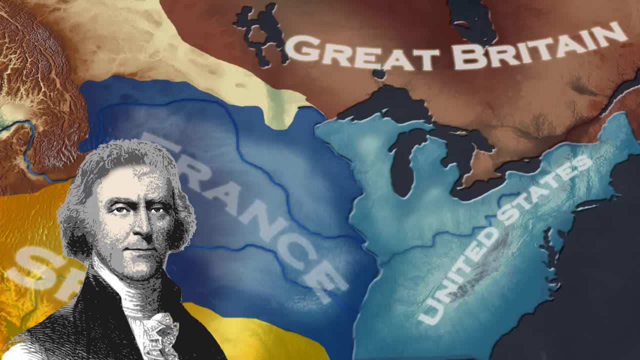 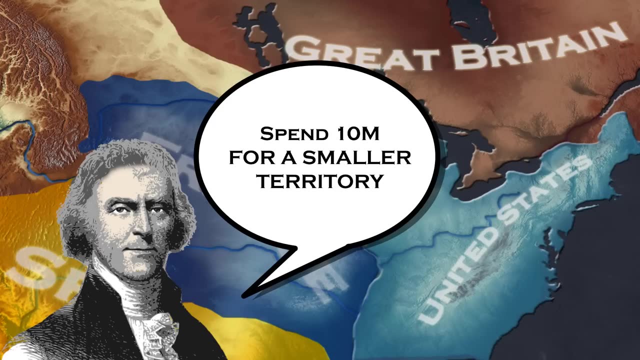 recognized And even so the American Revolutionary War. He bought the Louisiana Territory from France. Initial diplomats sent to France were allowed to spend up to 10 million US dollars in order to buy just New Orleans and, if possible, the West Bank of the Mississippi River. 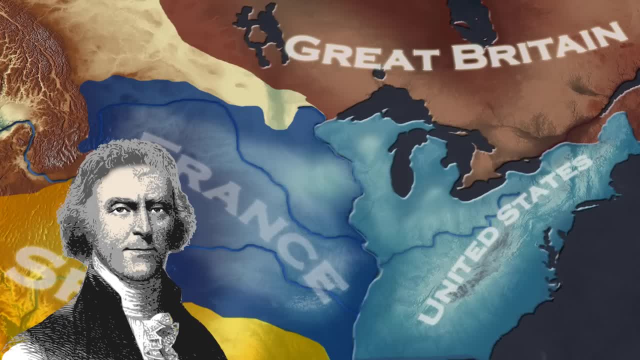 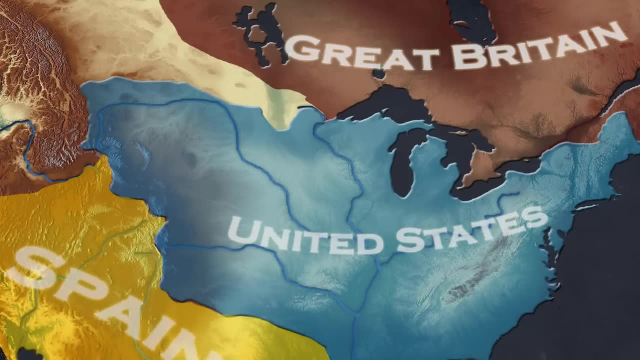 But the French government said that for 5 million more dollars all of the Louisiana Territory would be sold. The president approved the deal and the US doubled its size. In the middle of the 19th century some sessions were happening and Texas in joining the Union. 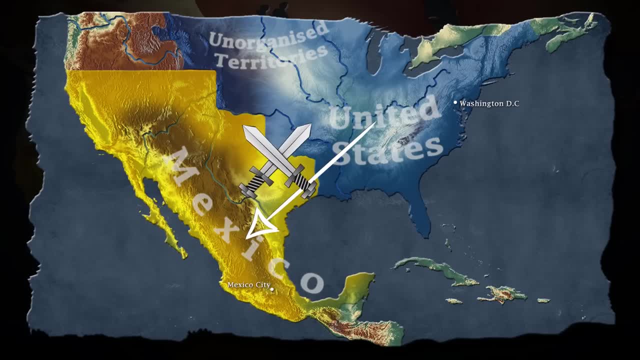 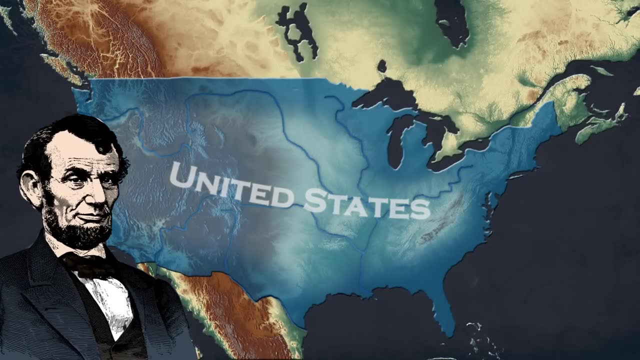 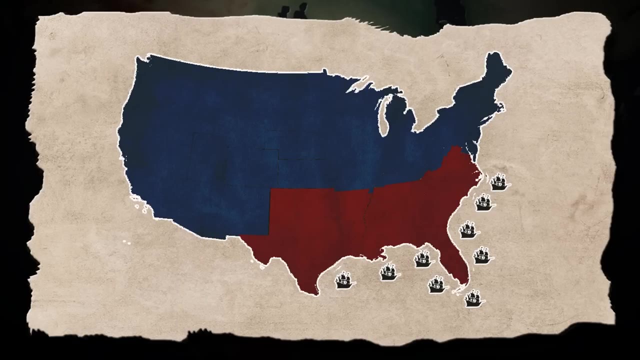 in 1845, and after the war against Mexican Empire, the United States will take important lands and expand even further. In 1861, after Abraham Lincoln was elected, some states from the South the Confederation attacked the rest. The South Revolt was happening due to controversy over the 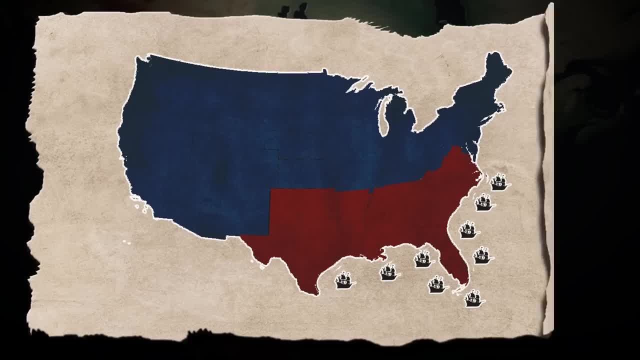 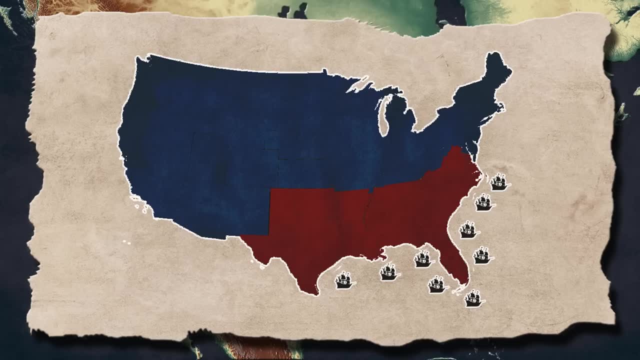 enslavement of black people. In 1860,, the United States was led by Abraham Lincoln, supporting banning slavery in all territories. War broke out in April 1861, when society of the United States and the United States of America were at war with the United States. 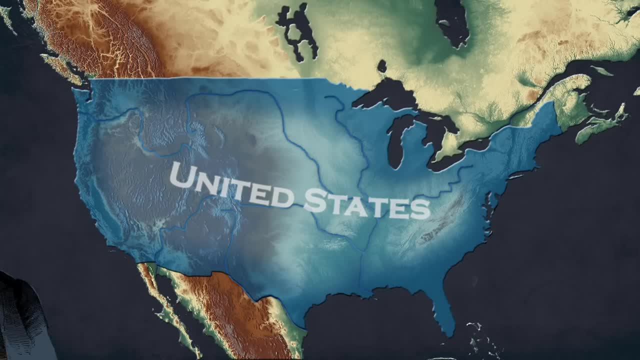 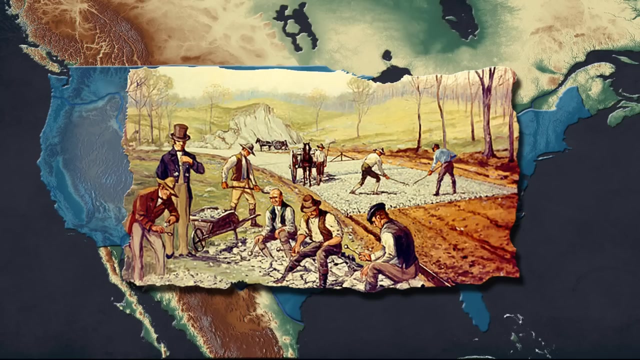 After four years of war, the Union achieved its victory and the Confederates were defeated. National unity was slowly restored. The national government expanded its power. The 19th century was a period of economic expansion. More and more industries were created and also the ascent was put on infrastructure. In 1898, the American-Spanish 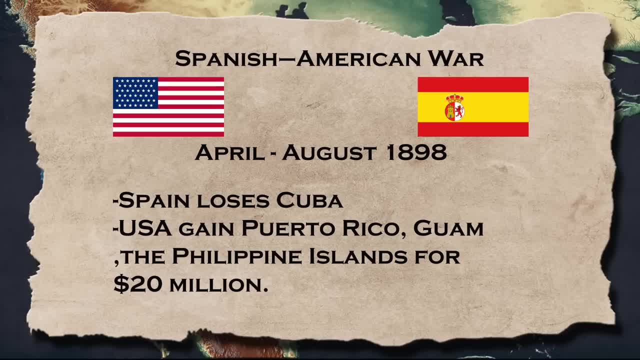 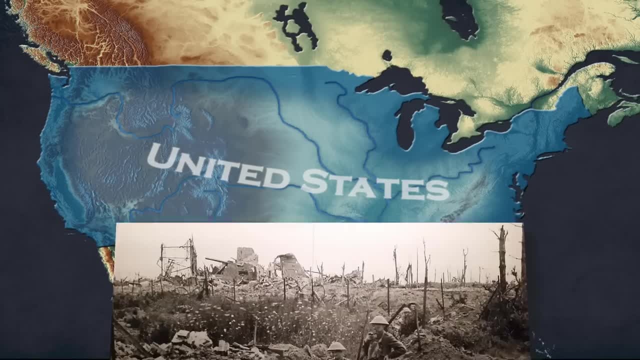 War is happening. Americans are winning in short-term some battles and at the Treaty of Paris the United States is getting the Philippines, Puerto Rico and Guam. At the beginning of the 20th century World War, I started Even though the United States was neutral. due to German attacks on the American ships and due to their intentions to make Mexico join against the United States, the Americans joined the allies. After this event, the economy was growing and all was good until the Great Depression which started in 1929.. 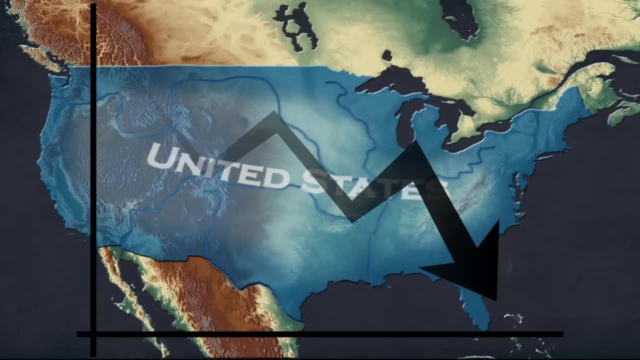 This event shook the world and created a base on which the Second World War will start. United States is getting the Philippines, Puerto Rico and Guam At the beginning of the 20th century World War. I started Even though the United States was neutral due to German attacks on the American. 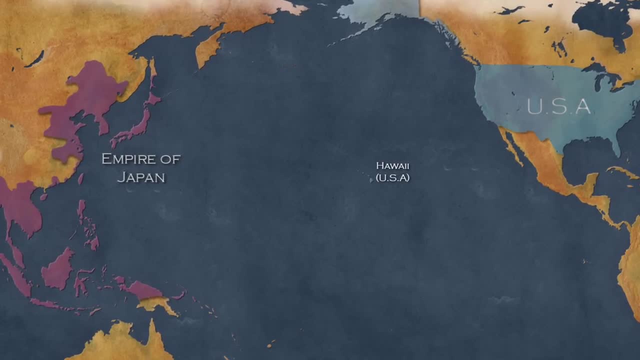 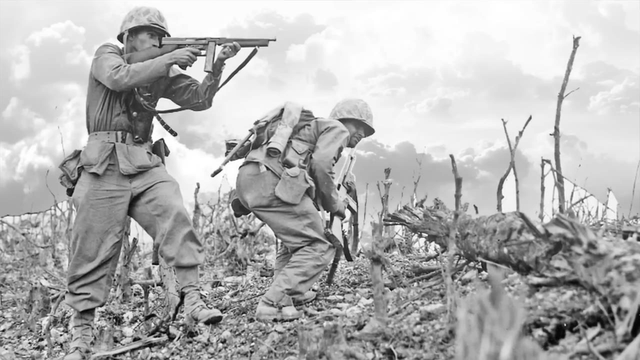 ships and due to their intentions to make Mexico join the United States, the Americans joined the allies. after being attacked at Pearl Harbor on December 7th 1941 by the Japanese Empire, Americans fought a distant war in Europe, Pacific and they provided supplies to the Soviets. 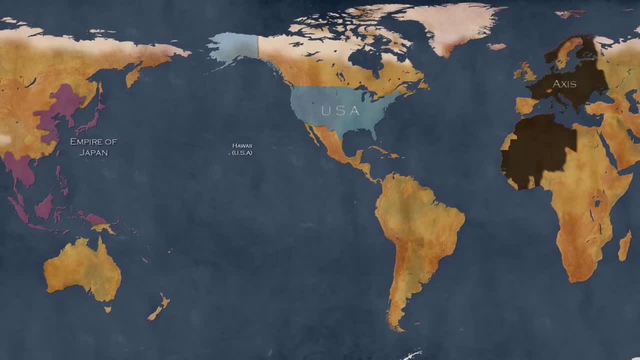 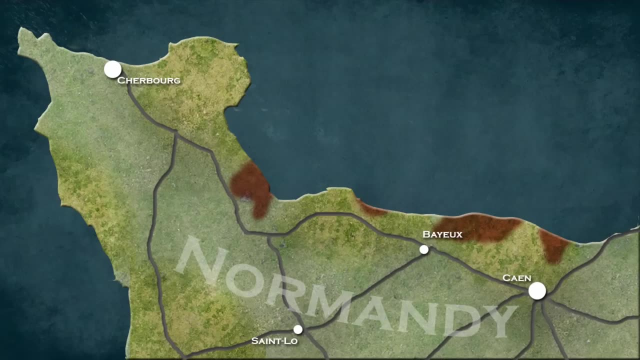 armored cars, motorized equipment, food, etc. Winning battle by battle in the Pacific, getting closer to the Japanese mainland, and after D-Day in Europe in 1944, the Americans managed to have a great impact and to help a lot on the Allied side. The war ended in.